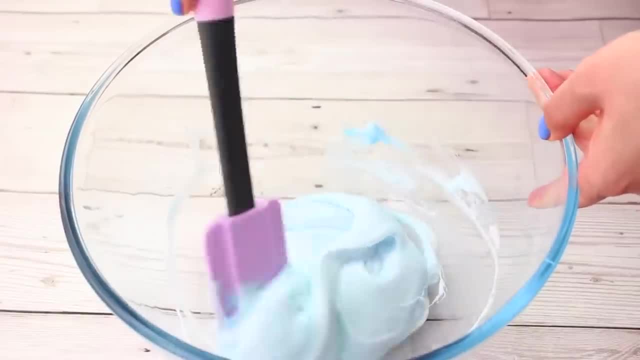 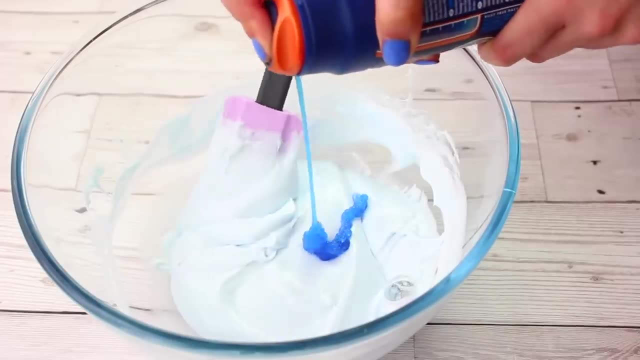 And it was just amazing. It kind of turned even fluffier than it would if I used the shaving foam And, as you can see here, the slime kind of started to pull away. and I googled it and apparently with clear slimes shaving foam actually works as an activator. 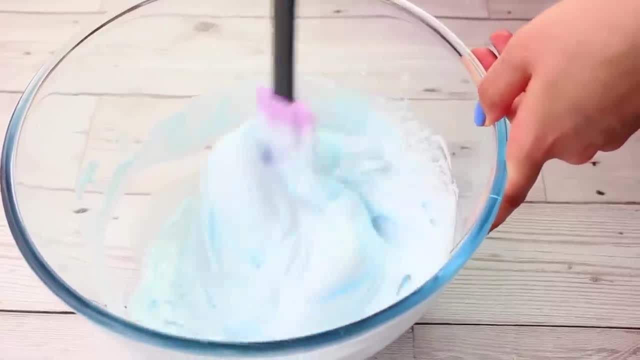 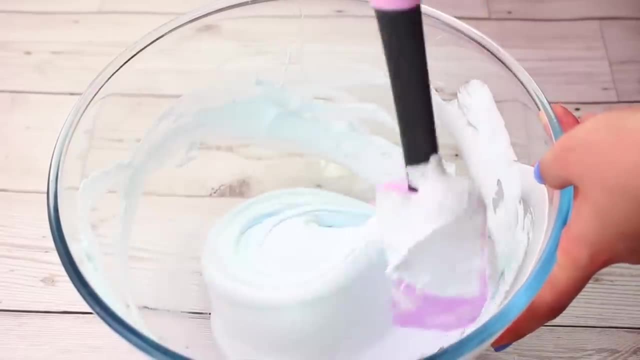 So I added a tiny bit more and it did pull away, but not that much. So I thought maybe I didn't add enough face mask and I went back in with a couple of packets and I think I added about 3 more and this just made the mixture a bit thicker. 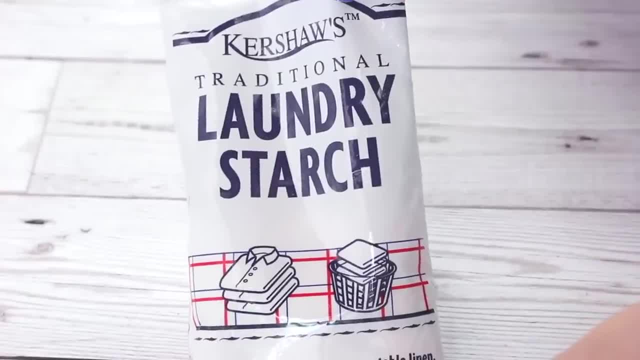 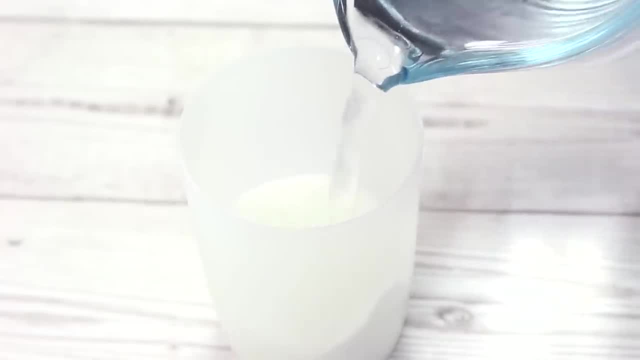 It did activate a bit, but not fully. So I decided to go in with Kerstle's Laundry Starch for an activator And I did 2 teaspoons of this and then I added some cold water. You can add hot, but personally I just like to add cold. 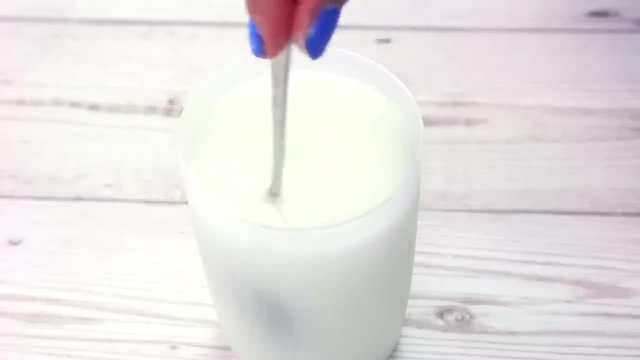 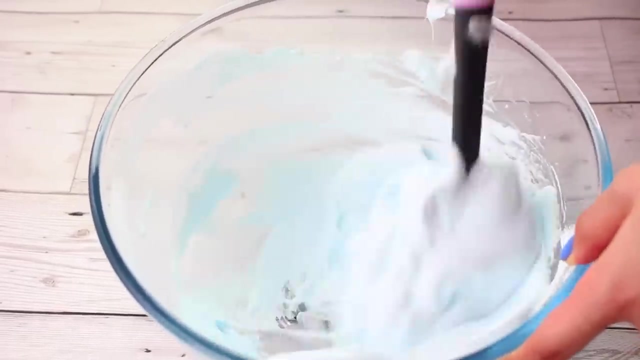 And then you just stir it up and you can't let this one sit, otherwise it all sinks to the bottom. so you have to do it quite quickly And I just add this in little by little and it activates very quickly, As you can see here. it kind of becomes hard, but the more you stir it it just becomes a bit more sticky and more slime-like. 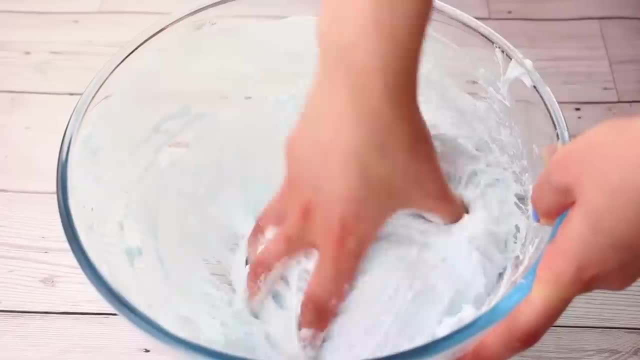 When the slime becomes difficult to stir, I just go in with my hands and start playing with it, And normally at first it's quite tough but then, the more you play with it, the softer it becomes and obviously the heat of your hands warms up. 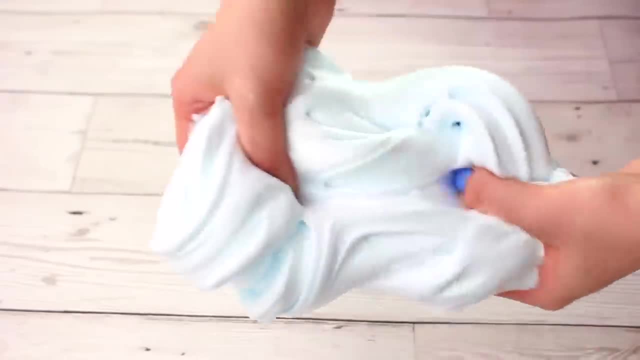 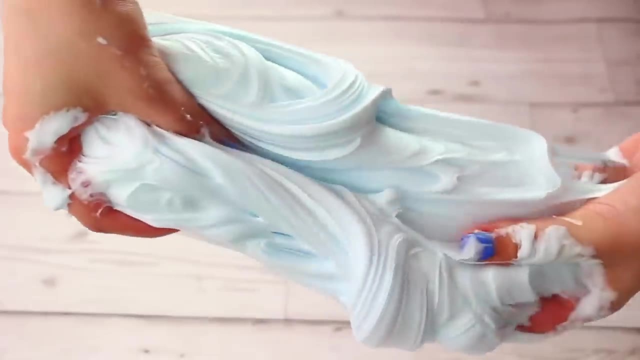 And it kind of melts the slime a bit so it becomes super fluffy and super stretchy, like this. I found that the slime didn't deflate at all. it literally kept its shape for so long. it was so soft and so stretchy, and I just absolutely love this method. 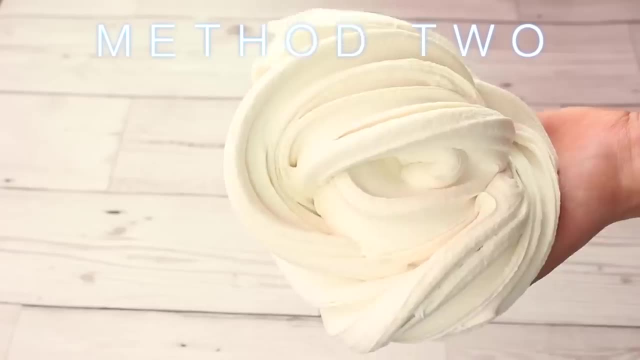 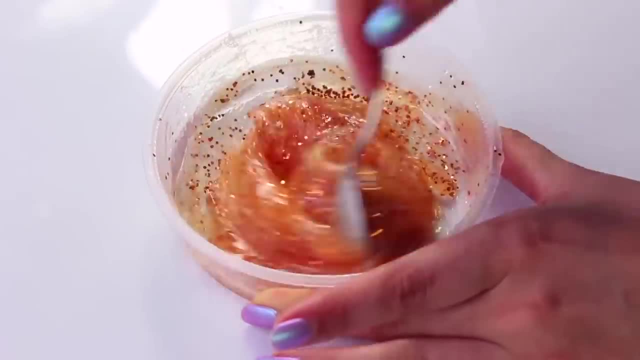 The slime normally comes in a little bit thicker than the previous method, but it's super stretchy and I just absolutely love this method. But for some reason, adding the water in really helped and, as you can see, this pretty much forms a slime. 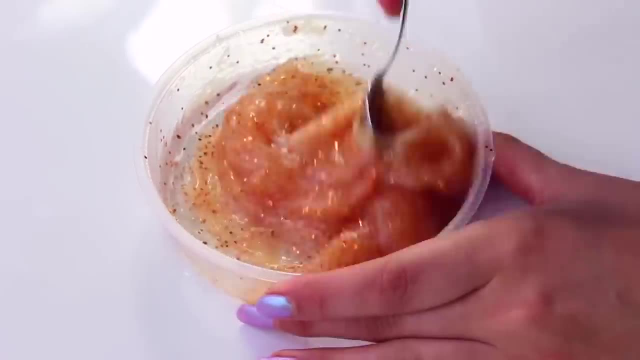 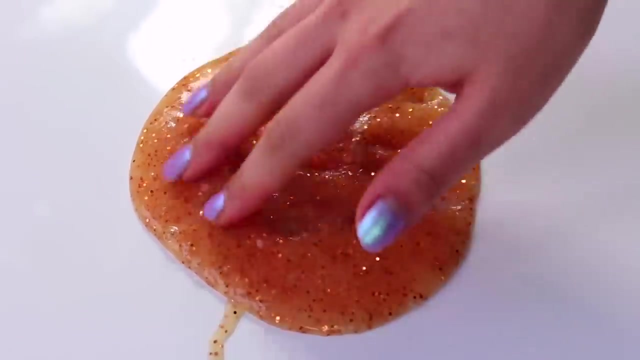 Like this looks amazing. I've never seen a no-glue, no-borax method pull away just like a slime. so I was so impressed by this And I decided to pour it out to see how it behaved, and it kind of fell like a slime, in that it was super thick. 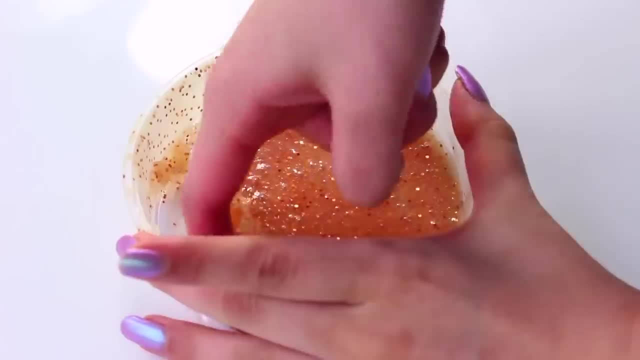 it didn't hold together and when you played with it it still was very sticky, but you did get some clicking sounds. To try and get rid of some of the stickiness, I put it in the freezer, but this changed the consistency completely. 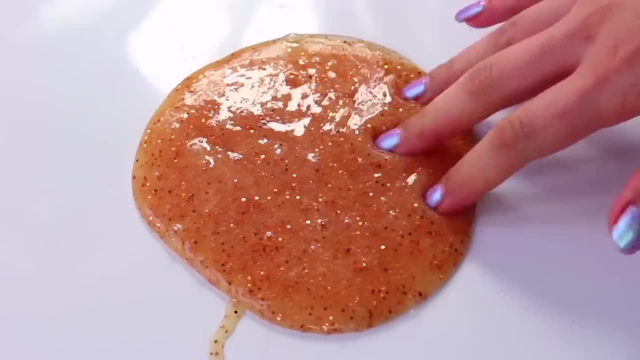 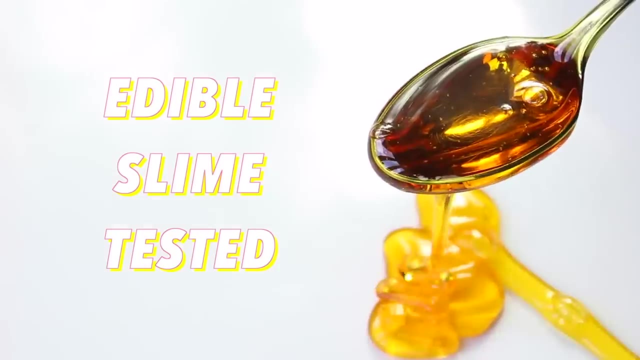 so I really don't recommend doing this. It just kind of became like a big bogey, But I'm going to be testing out some popular edible slime recipes and I really hope that you enjoy it. So first up, we have marshmallow slime, and I'm using some mini marshmallows from this. 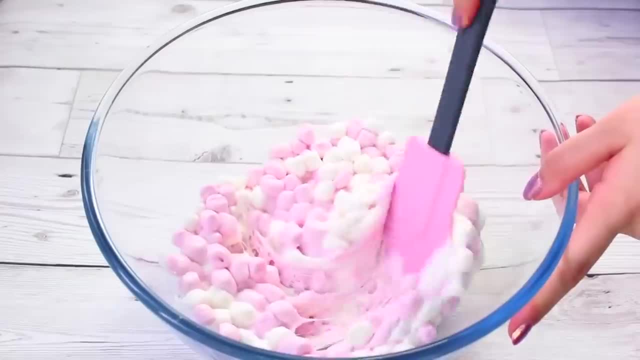 I think you can get it from any supermarket in the baking aisle, And then I just put it in the microwave for 10 seconds on the lowest heat setting. Once everything's mixed in, it'll be pretty sticky, so we're gonna use some icing sugar. 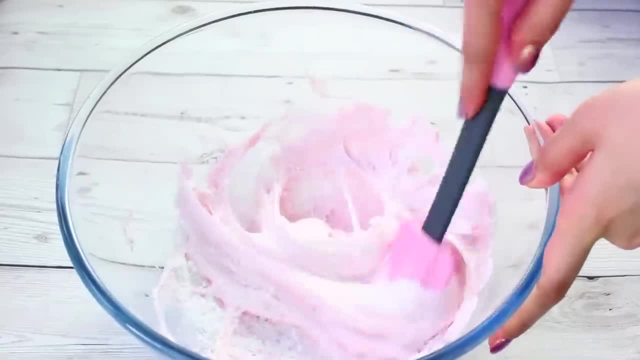 and I think you guys in America call it powdered sugar- just to make it lose some of the stick and pull everything together, And I found that it became super slimy at this stage. and I also found that it became super slimy at this stage. and I also found that it became super slimy at this stage. 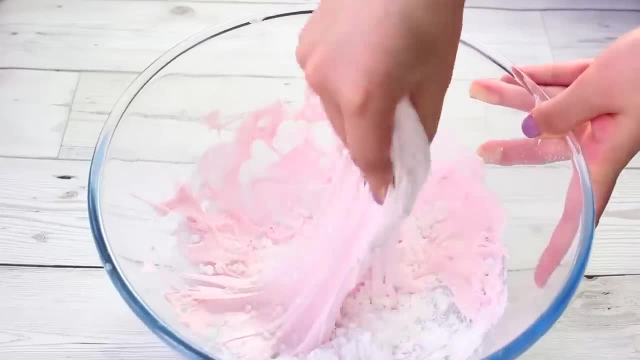 and I also couldn't really mix it around with a spatula anymore. so I waited for 10 minutes to make sure it was cool and then, once it was, I just went in with my hands and started mixing in the icing sugar this way: 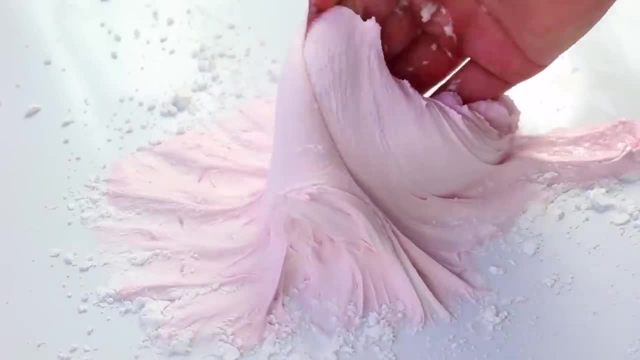 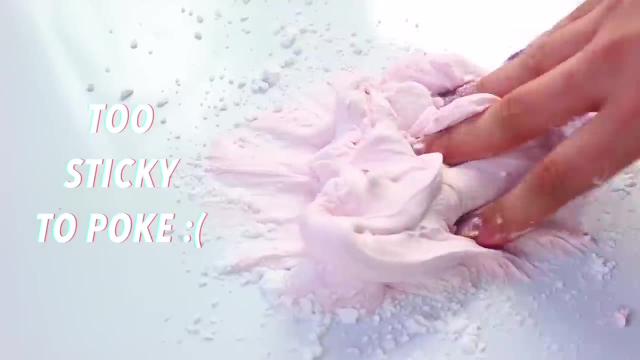 and, as you can see, it's so stretchy and slime-like. The only bad thing about this method is that it stays so sticky and you can't really poke the slime because of this. The next slime we're going to be testing is golden syrup slime. 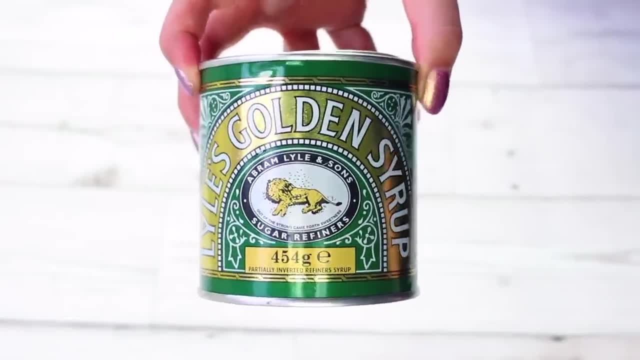 and I really love this because it's so pretty when it's being poured out and, as you can see, it's so pretty when it's being poured out and, as you can see, it literally looks like golden liquid and it's kind of like a thicker version of honey, I guess. 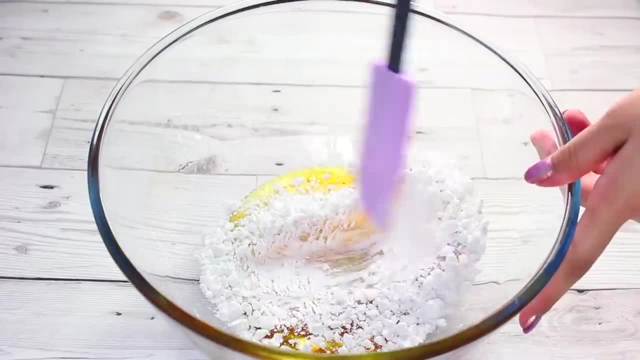 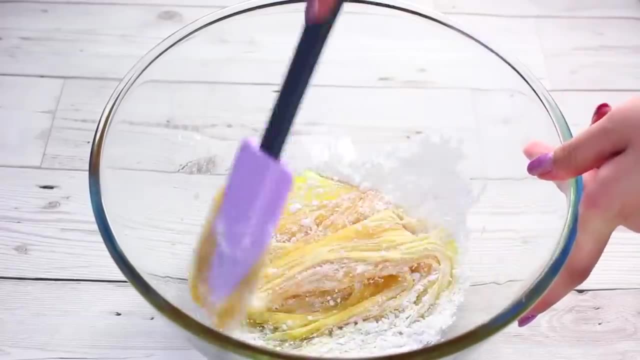 and it smells so good just like toffee, and I decided to add a tiny bit of powdered sugar, because this is such a thick mixture that I didn't think it would need much, and I was so, so wrong. The first batch of sugar that I mixed in didn't actually make much of a difference. 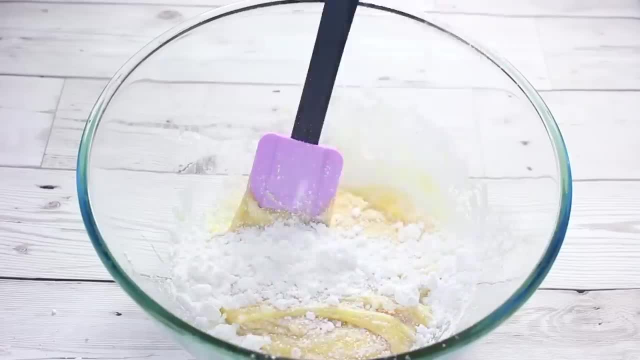 so I started to add loads and loads and I think I actually added the whole box before it actually worked and it kind of became like a dough. so I was really worried and I decided to go in with my hands, and obviously this one isn't hot. 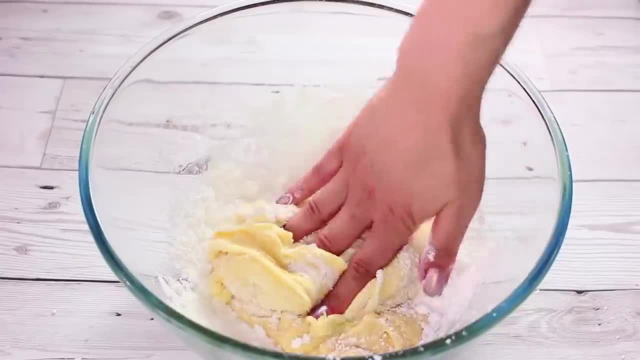 so you can go in with your hands at the start if you'd like to, but personally I thought that would be too sticky. and with the final bits of icing sugar you don't want to add too much so that it becomes a dough. 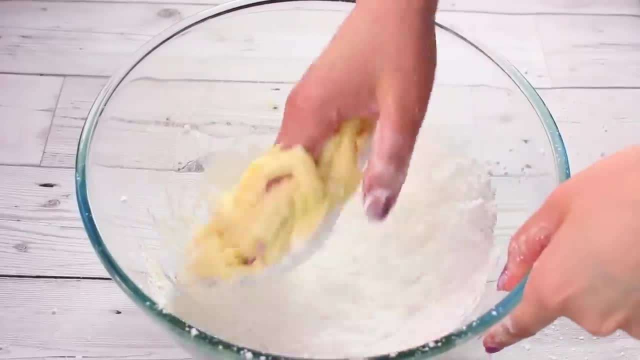 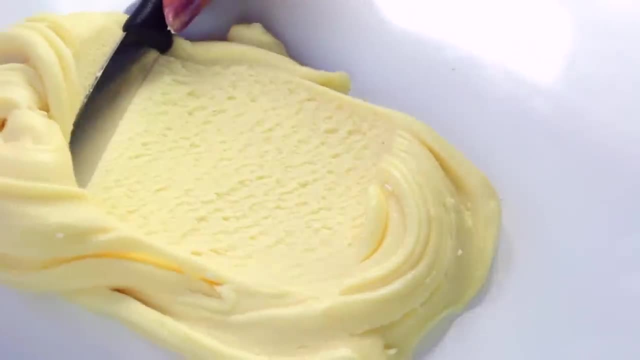 so what I like to do is just dip it in the icing sugar and play with it in my hands, and the heat of your hands will melt it a bit. so even if it is a bit too hard, it can be saved and, like you can see here, it literally turns into a butter slime. 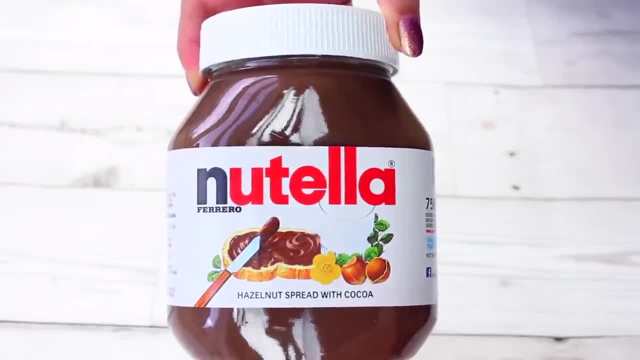 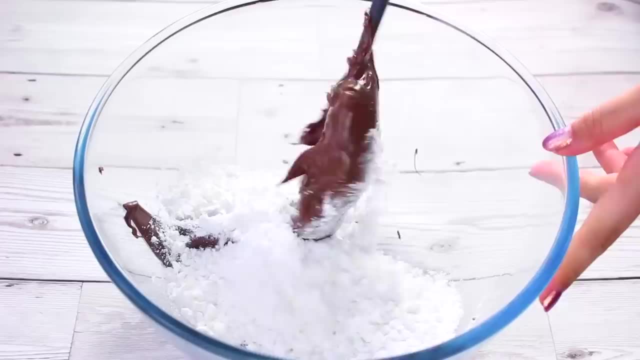